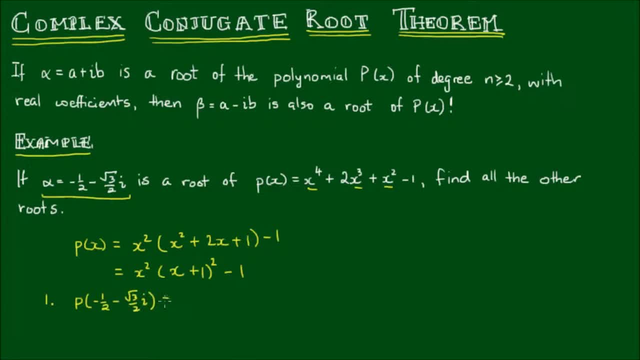 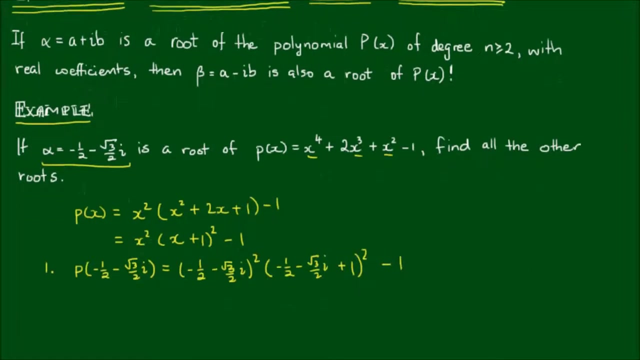 root 3 on 2i gives us the answer of zero. So we evaluate a half minus root 3 on 2i squared by a half minus root 3 on 2i, plus 1 squared minus 1.. The first squared term evaluates to minus a half. 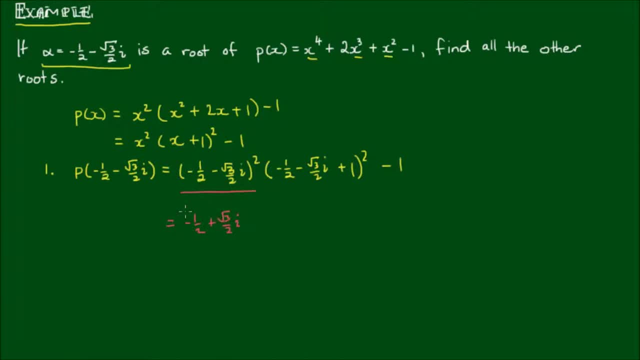 Plus root 3 on 2i, And you can satisfy yourself that this is the result. The second squared is equal to minus a half, minus root 3 on 2i, And we're left with the remaining term minus 1.. So here we have a case of complex conjugate multiplication. 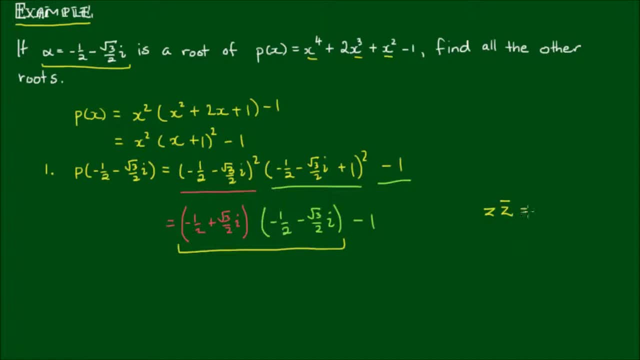 So z by z bar, And the result of this is: It's simply the real component squared plus the imaginary component squared, So we have 1 quarter plus 3 quarters minus 1, which of course equals 1 minus 1, which is equal to zero. 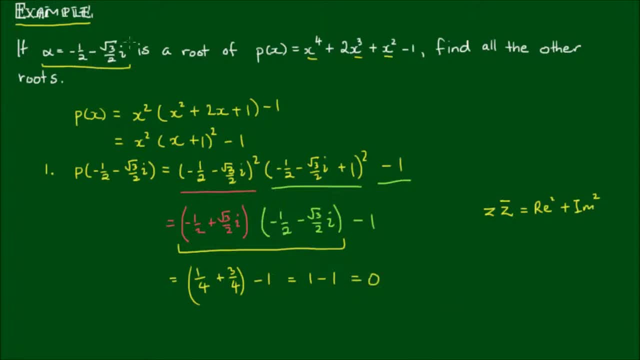 So therefore alpha is equal to a half minus root 3 on 2i is a root of p of x, And then by the complex conjugate root theorem we can say that beta is equal to a half plus root 3 on 2i is also a root. 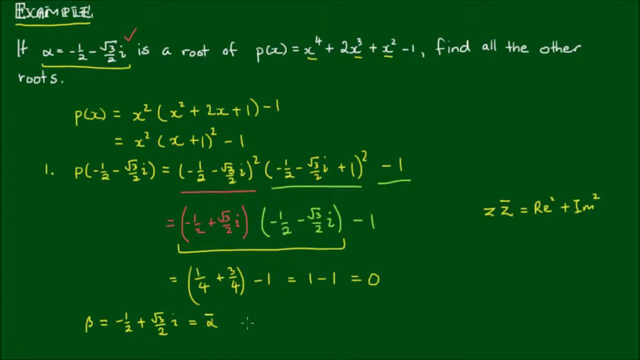 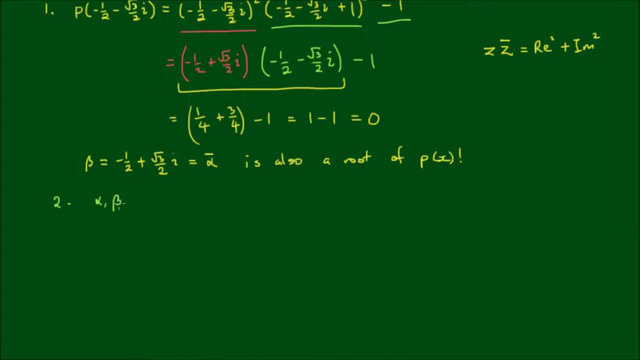 So beta is simply equal to alpha bar And it is also a root of p of x. Okay, now that we have the roots alpha and beta, then x minus alpha and x minus beta are factors of the polynomial px. So if we then expand this expression, so we get x squared minus alpha plus beta, x plus alpha beta. 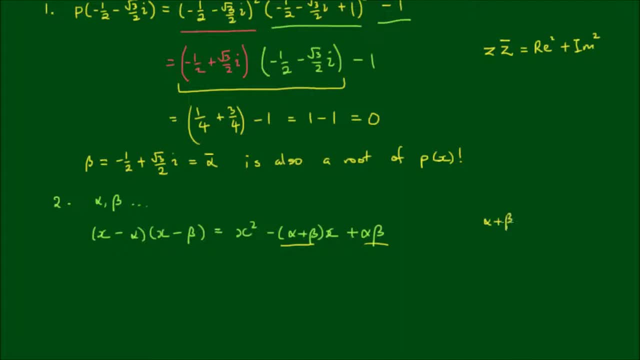 And let's evaluate each of these components. So alpha plus beta is simply a case of z plus z bar, which is equal to 2 times the real component, which in this case is a half negative, a half times 2,, which is equal to negative 1.. 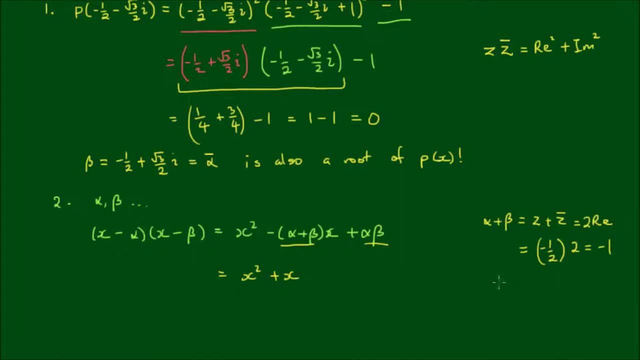 So we get x squared plus x And alpha times beta in this case is a case, another case of z times z bar, And we know the results of this. So the real component squared is 1 quarter and the imaginary component squared is 3 quarters. 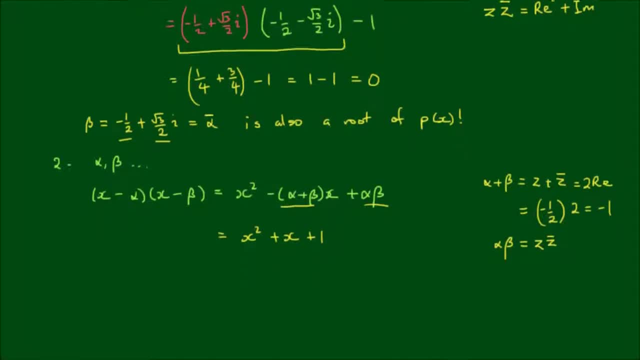 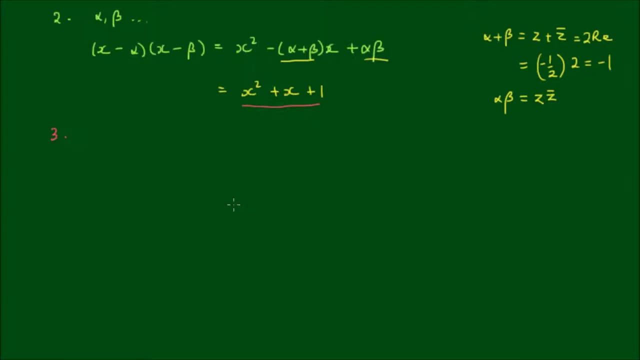 So 1 quarter plus 3 quarters is equal to 1.. Now let's divide p of x by this factor: x squared plus x plus 1.. So p of x is equal to x to the fourth plus 2x cubed, plus x squared plus. 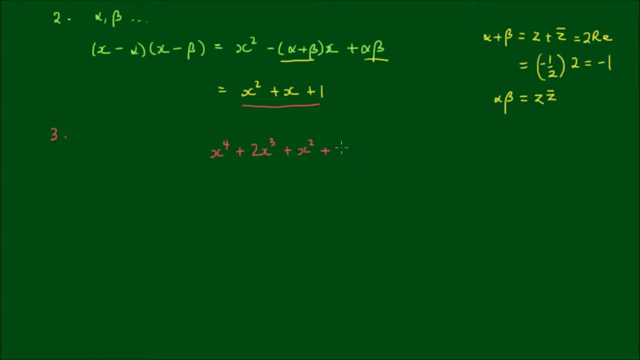 We didn't have a linear coefficient, but I'll put it down as a placeholder anyway. So we say 0x, then minus 1, and then we divide by x squared plus x plus 1.. So I need to multiply x squared by x squared to get x to the fourth. 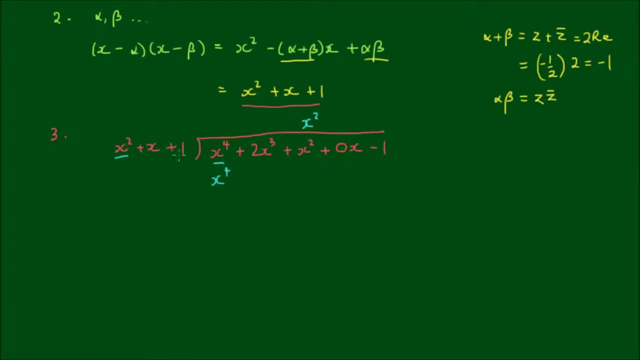 So x squared by x squared is x to the fourth, x squared by x is x cubed and x squared by 1 is x squared. And I take the new line from the line above and I end up with x cubed plus 0x squared. 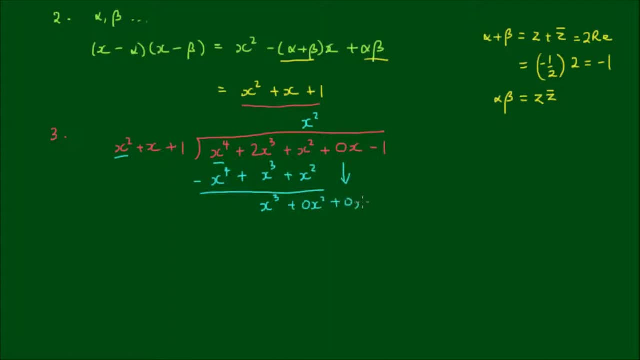 And then we bring down the 0x, To get x cubed I need to multiply by an x, So x by x squared is x cubed plus x squared plus x. And I subtract the new line from the line above to get minus x squared minus x.